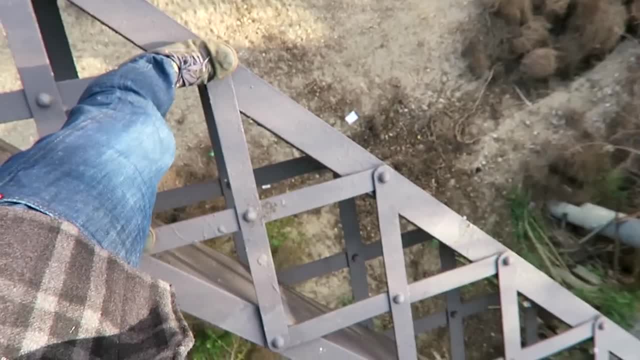 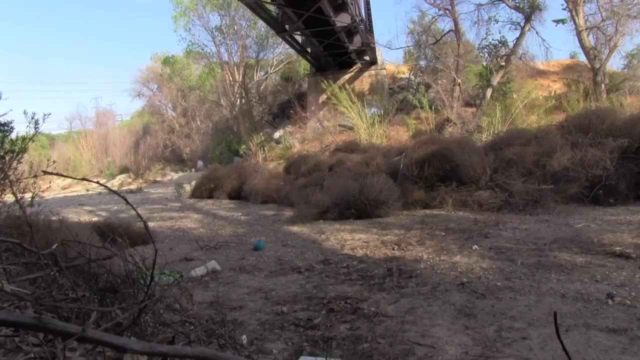 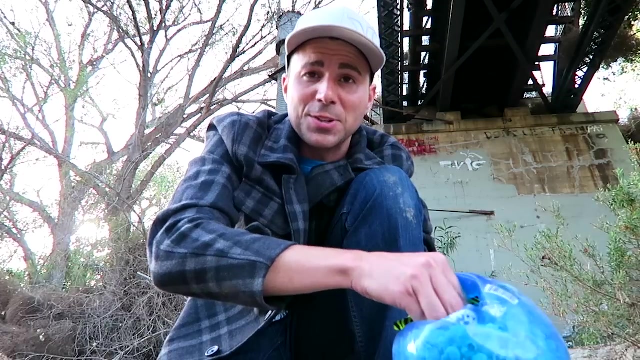 I'm using a ball here because it's more weight efficient than a box, where you have unnecessary cushioning in the corners. plus, the stretchiness of the ball will help absorb some of the energy. The moment of truth, and we have an intact egg. Now, before I show you the other four ideas, let's 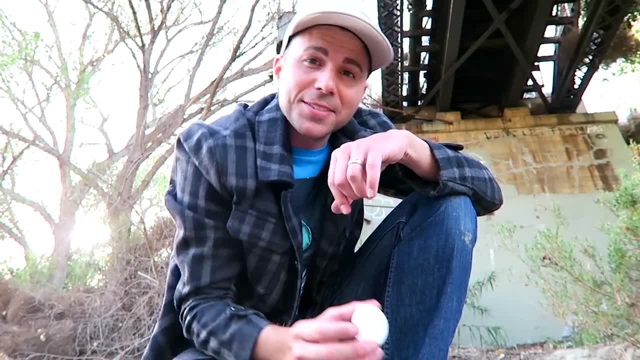 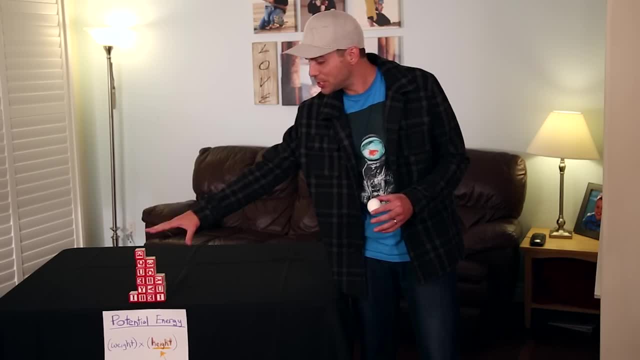 talk about the science behind landing with an uncracked egg. So at the start of your drop your egg is up high and it's stationary, so it has potential energy, which is the energy associated with height. So these red blocks represent the potential energy, and the higher I go, 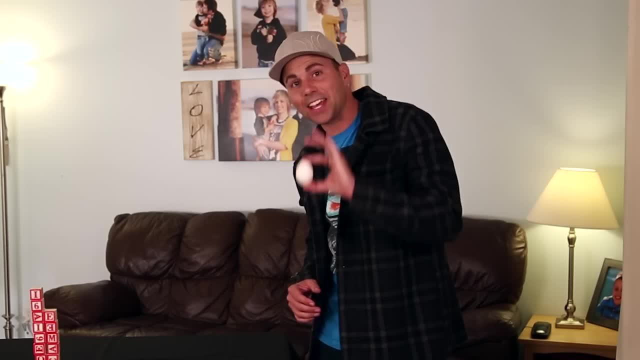 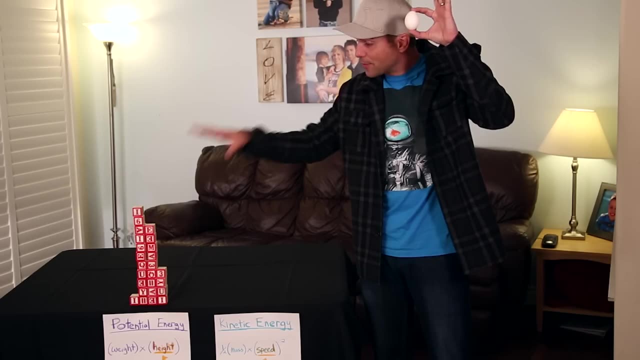 the more blocks of energy I start with And then, as the egg falls, that potential energy is converted to kinetic energy, which is the energy of speed. So you start up high and every single block is over here as potential energy. but as you start to fall and fall faster and faster, every single block. 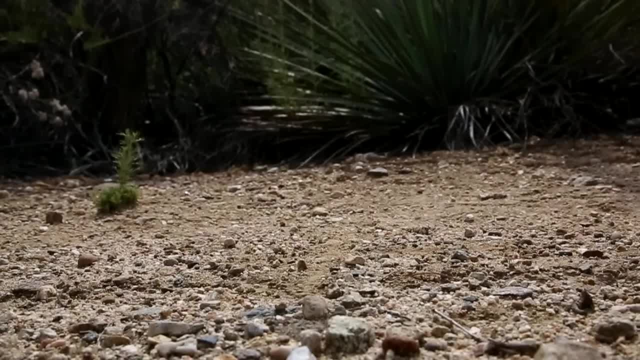 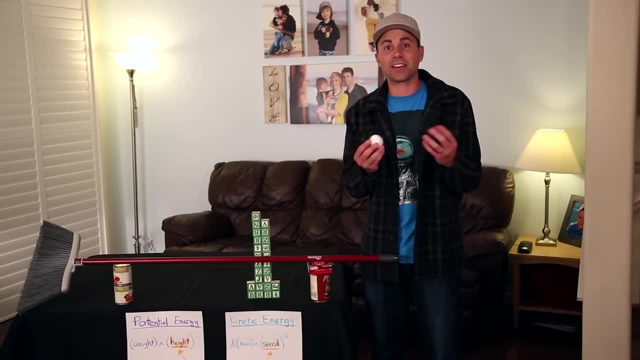 comes over here as kinetic energy or speed. And now your egg is about to impact the ground and has all this energy in the form of speed that it's got to go somewhere. Now. this broom represents the standing energy that holds an egg shell together and makes it hard. So the way to think about this. 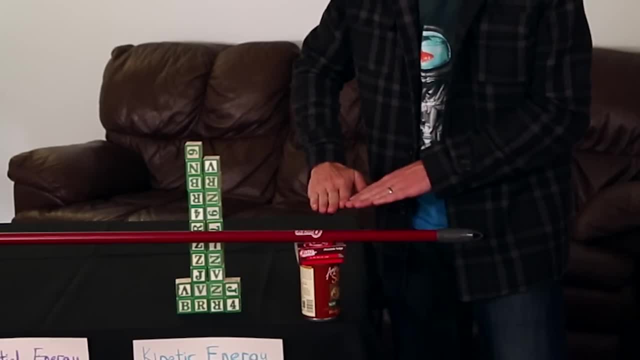 is when your egg hits the ground. if you introduce more energy than the binding energy of the egg, you're going to have more energy than the binding energy of the egg, The binding energy of the molecule holding the hard egg shell together. at any point you're going. 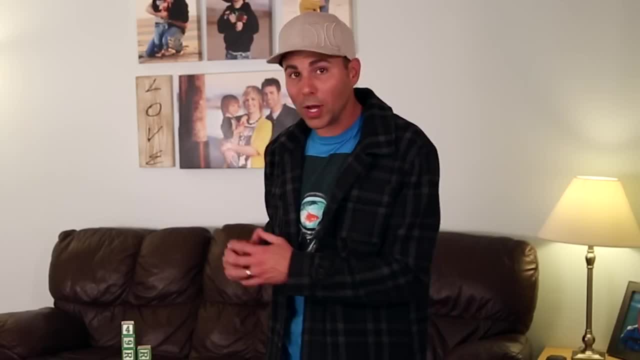 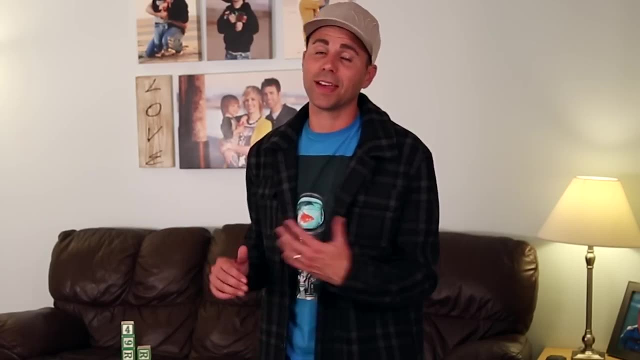 to break at that point. So the question then becomes: what can we do to keep our blocks below the broom? because, simply put, below the broom your egg is safe. Anything above the broom, and your egg is busted. Well, there's two things we can do. The first is that we can make this pile of green blocks. 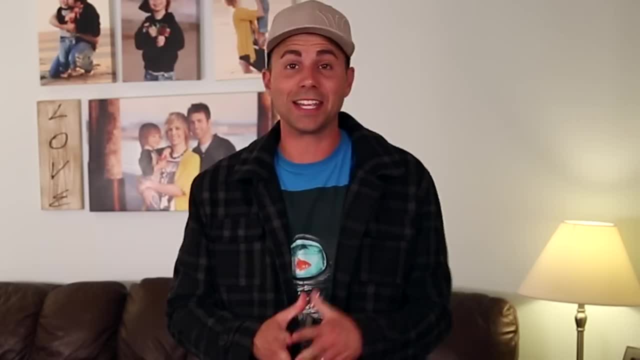 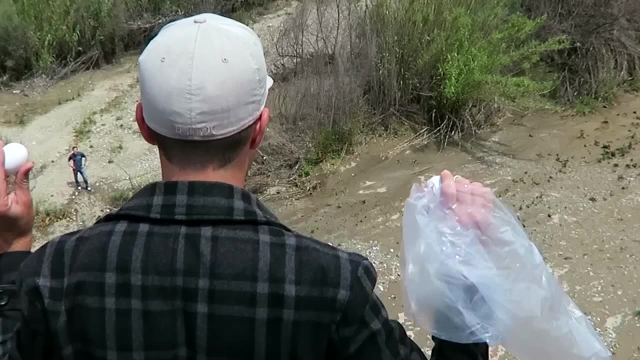 not as tall. This is why, no matter what your contraption is, to protect the egg, if your rules allow it, you should make a parachute, The bigger the better, and it does not have to be fancy. This is like old school army guy style: just cut up a trash bag, a little bit of string, a little bit of tape and just 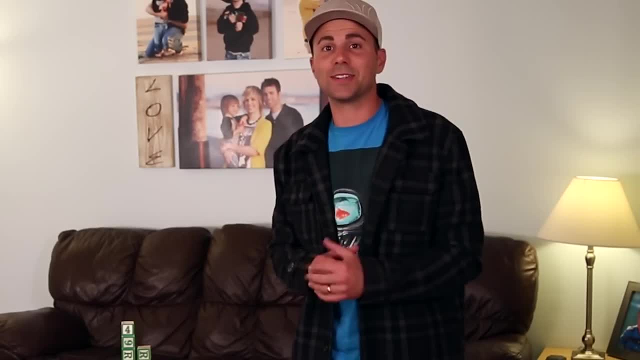 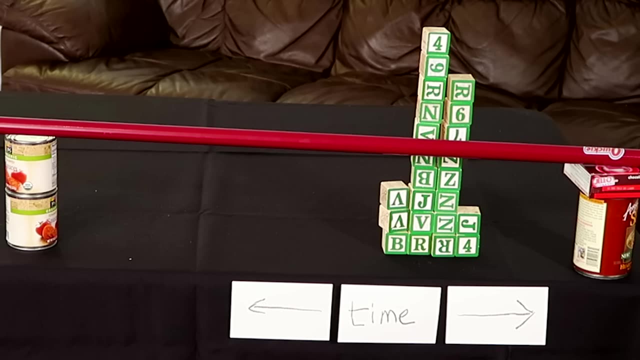 looking at this, you can see the difference a parachute can make. So the second thing you can do is not to remove any green blocks by reducing your speed, but to spread them out. So if we say left to right is our time axis, the more we can stretch out this impact event, the more we can. 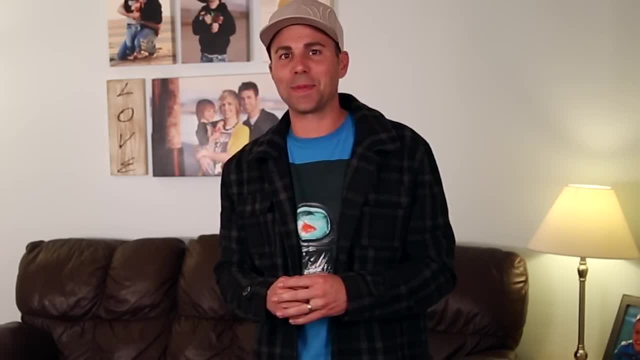 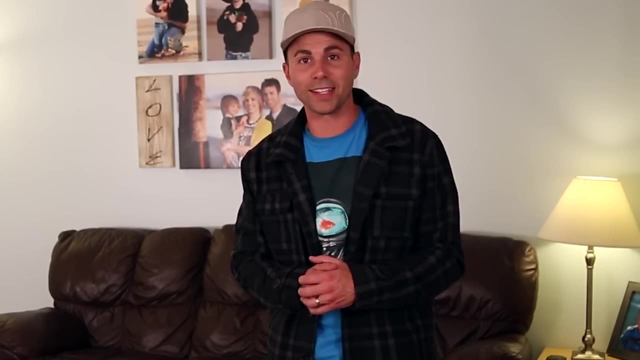 lower that high energy spike. And this is a cool way to think about any two objects impacted: The longer the duration of the impact, the more you can spread out that force so stuff doesn't break. So, for example, this is a cool way to think about any two objects impacting: The longer the duration of the impact, the more you can spread out that force so stuff doesn't break. So, for example, 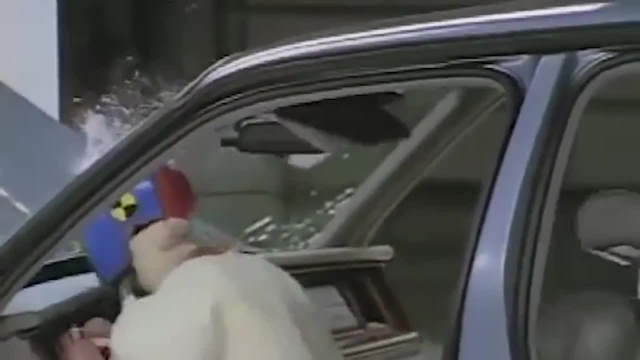 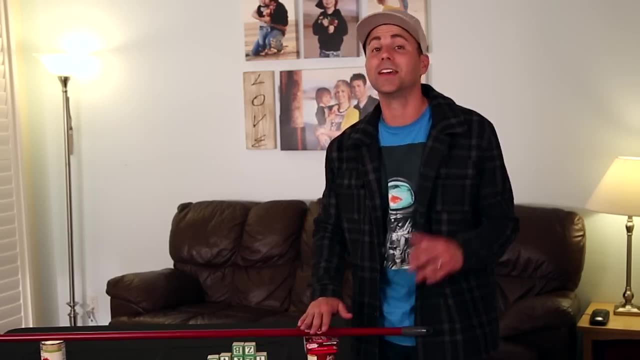 this is the point of car airbags: Instead of your head hitting the steering wheel and stopping near instantaneously, it stretches out the impact force over time, so you don't get a quick spike that exceeds the broom line for your skull. This is exactly why long jumpers prefer to land in sand and not on asphalt, and why parkour runners will. 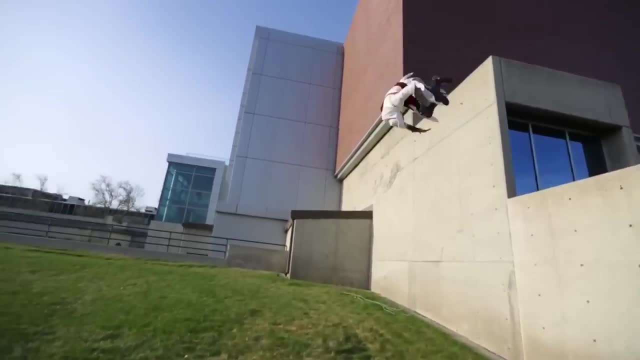 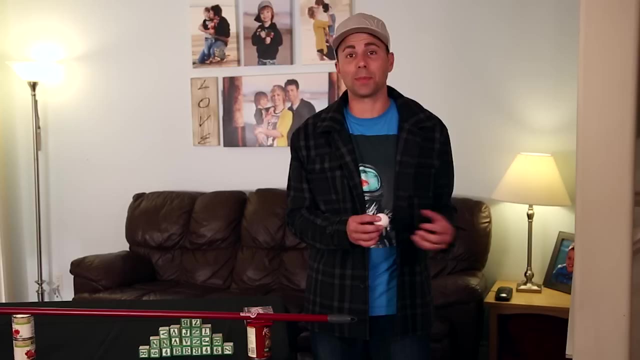 always roll after a big jump. It's all about diffusing the force over a longer period of time. So what does that mean for our egg contraption? It's really just something to keep in mind, because it can make it more intuitive, for example, to see why putting your egg in the middle of a jar. 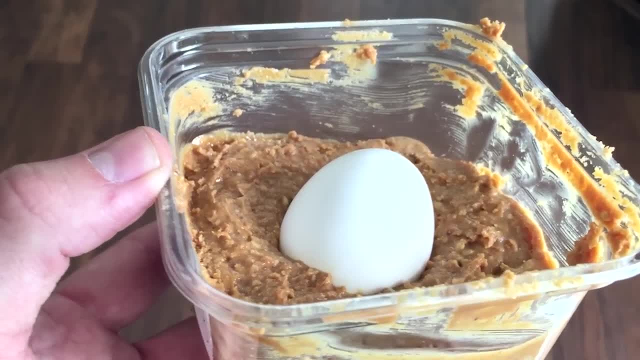 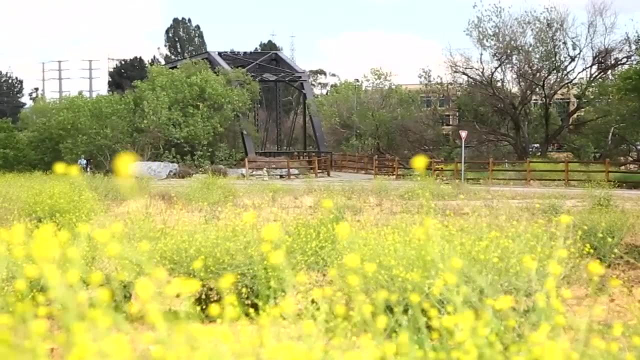 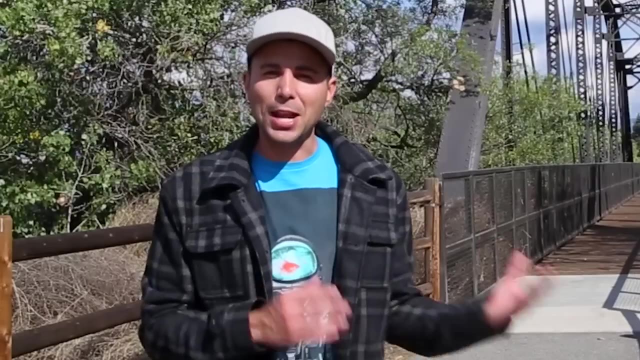 peanut butter, which is a popular and not a very good idea, isn't as good as putting your egg in the middle of a popcorn ball. Okay, back to the bridge. So a lot of people like to build contraptions out of straws, and in some competitions that's. 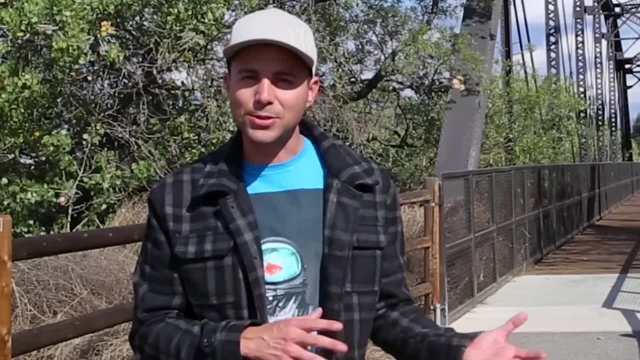 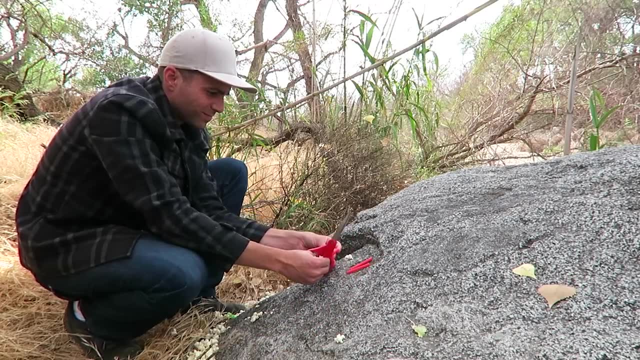 all you have to work with. How you configure your straws depends a little bit on how stiff they are. The good folks at Wendy's have fairly stiff straws, which means I didn't have to use quite as many. So my idea was to take six like three inch long straws and build a regular triangular. 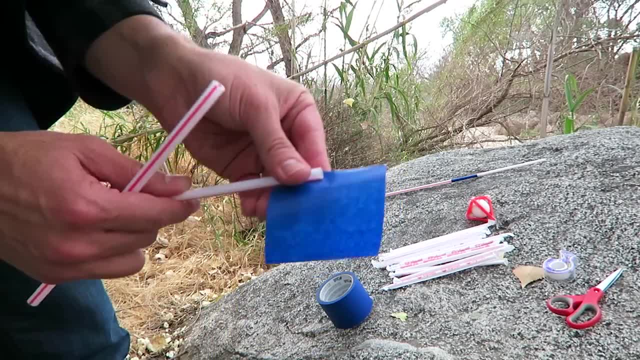 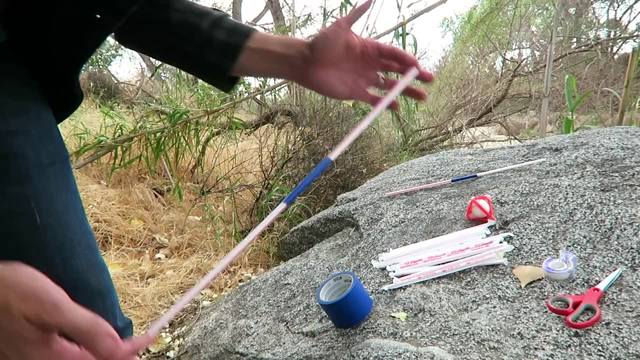 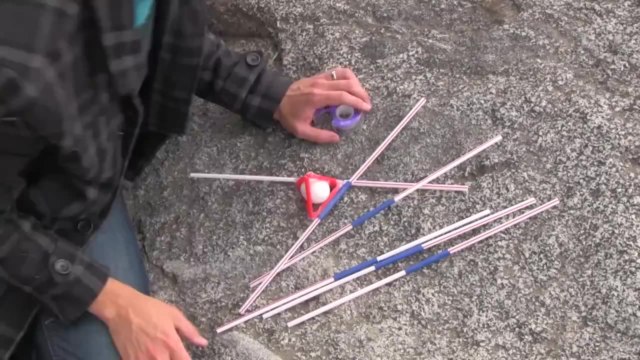 pyramid and then put the egg in the middle. And then I took two of the Wendy's straws and joined them together to sort of make a mega straw, and I used this white tape to help prevent it from buckling. And then I made six of those mega straws and simply taped one to each edge of the pyramid. 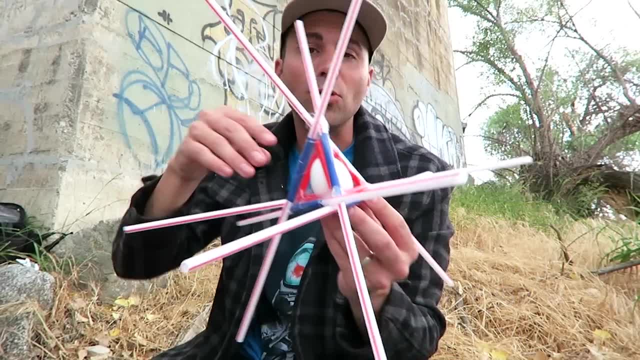 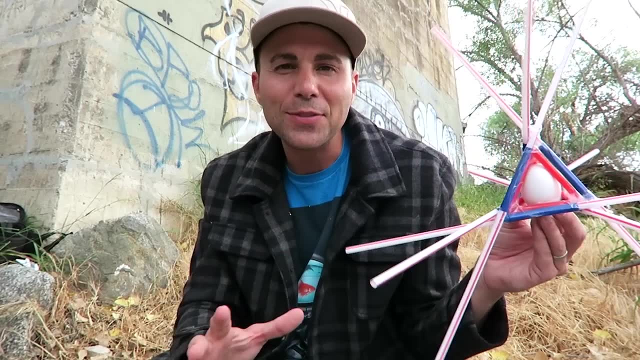 So the main point here is that there are no straws pointing directly at the egg. When it impacts the ground, the force goes up the stiffest path, through the straw. I saw a ton of examples online where the straw was actually pointed at the egg, which would 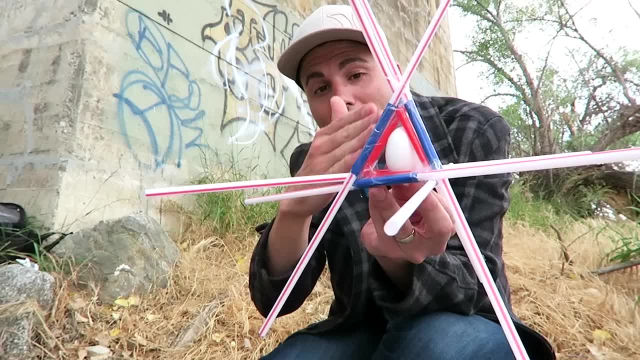 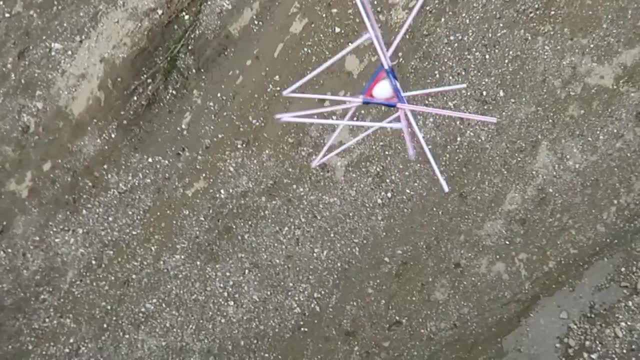 create a puncture load. In our case, we have this pyramid, so all the loads pass next to the egg, so you don't get that primary impact. Three, two, one, Okay, Okay, Okay, Okay, Okay Okay. 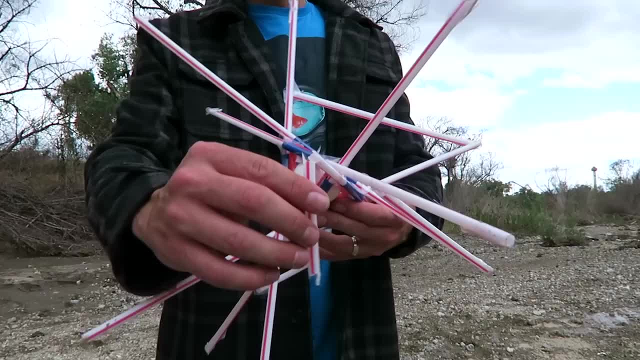 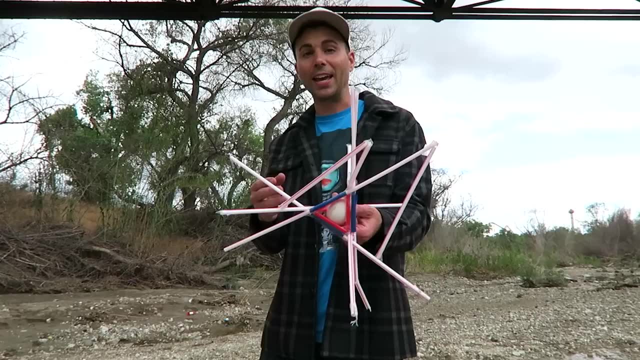 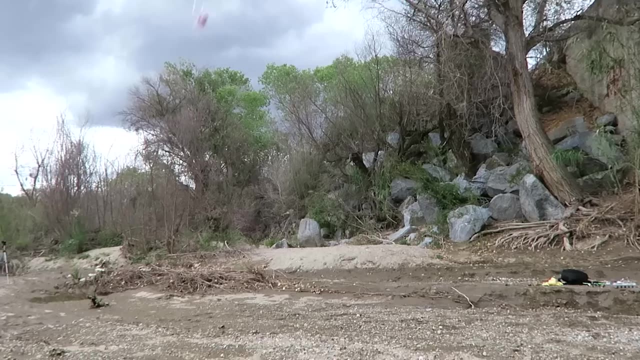 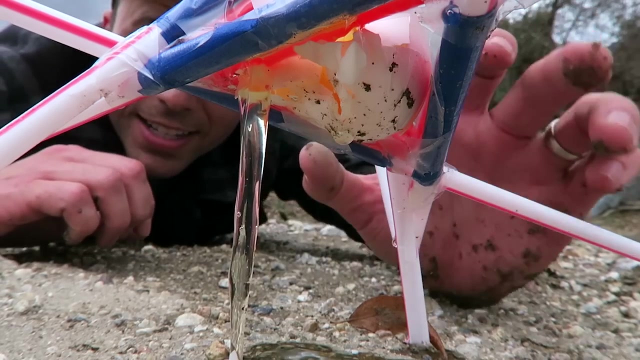 Okay. So you'll notice we've got a couple of broken pieces, but that's okay because it took energy to make those breaks and that served to protect the shell of the egg from receiving that energy. So success. Okay. so our egg finally broke, but it took about 20 tries and you can see there's a 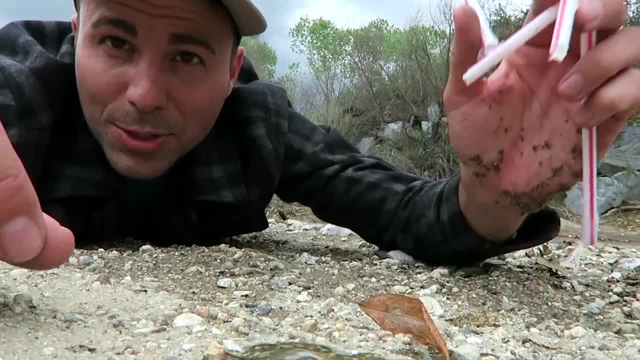 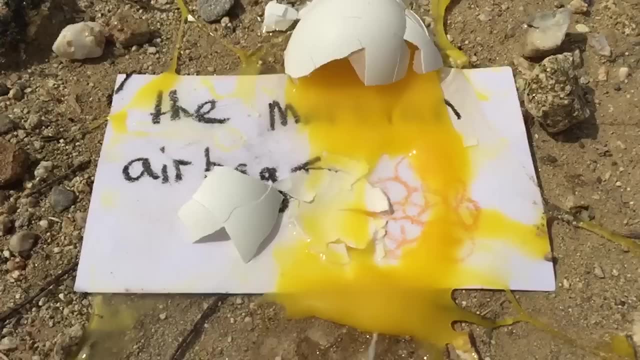 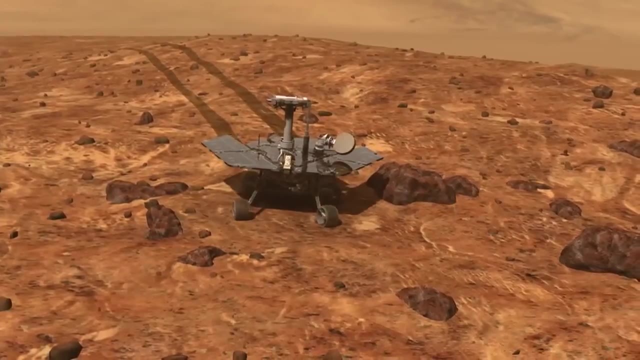 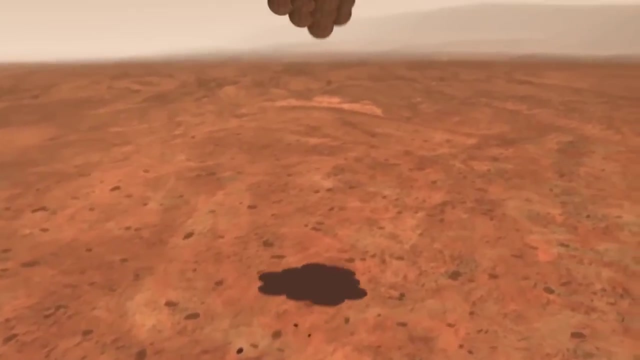 lot of busted straws here. All in all, it was pretty ridiculous. Resilient, yeah. So this one is a throwback to my NASA roots. in 2004, the mer rovers landed on Mars using giant airbags And even though Mars has one-third the gravity of Earth, I figured it would still work. I. 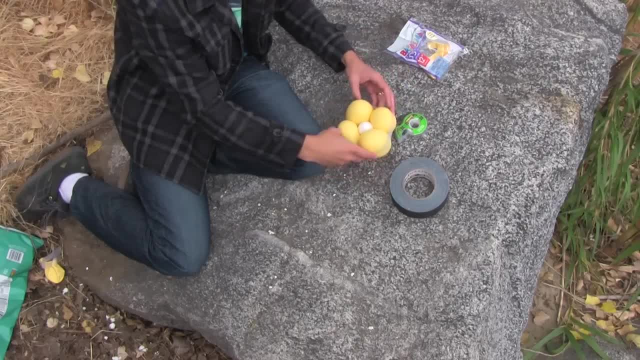 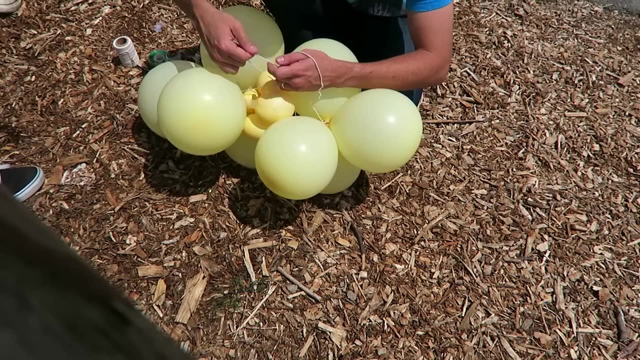 Started by cushioning the egg in four little balloons that I barely filled up, and then I blew up bigger balloons, Then just tied it all together with some string and tape and then, if there's any gaps in coverage, You can just tape a balloon directly to the string you just tied around. 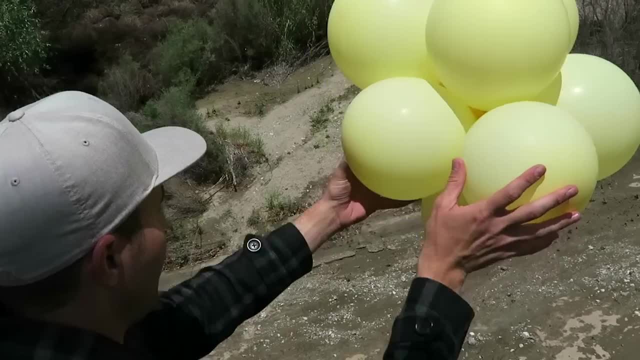 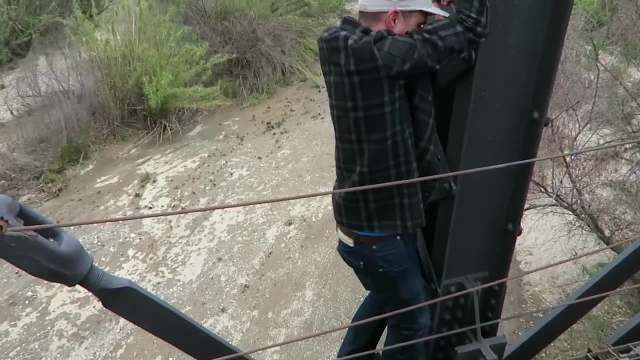 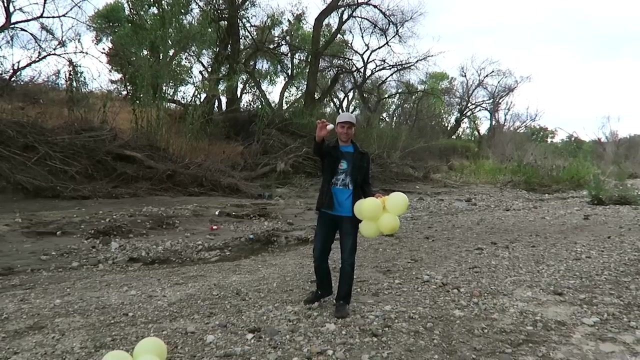 In addition to the balloons extending the impact time, this design benefits from a large cross-sectional area relative to his weight, So in a sense it becomes its own parachute. Of course, if your rules allow it, you should still throw an additional parachute on it anyways. Touchdown confirmed. 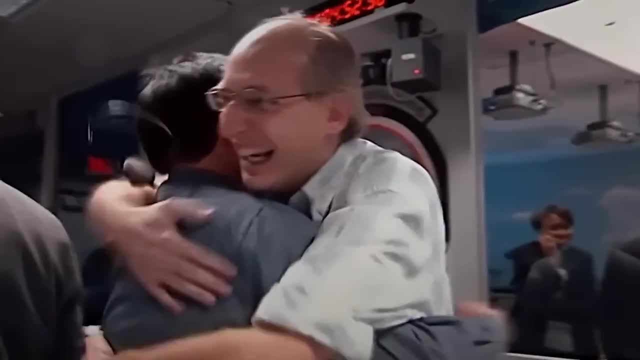 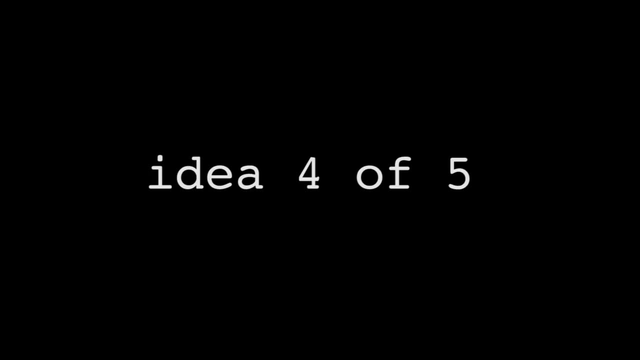 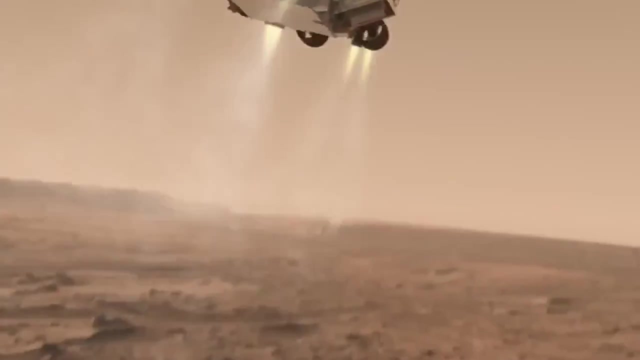 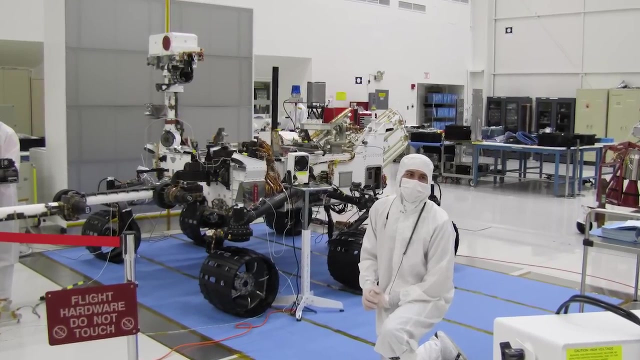 On 2012, we landed another rover on Mars called curiosity, but this one was too big to use airbags, So we had to have a power descent, pretty much like a jetpack. So I wanted to pay tribute to curiosity, since I got to work on her for seven years and at first I was thinking like: 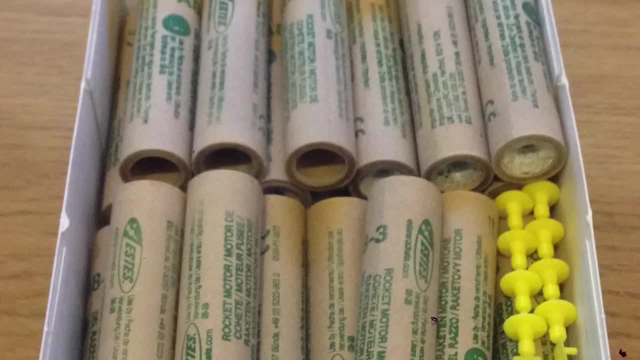 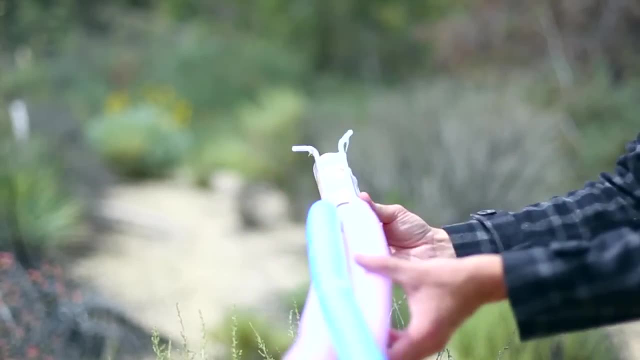 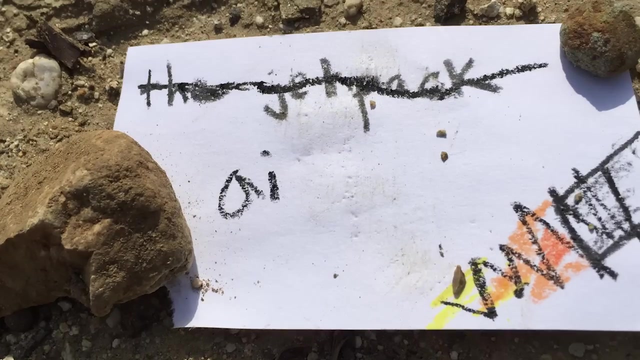 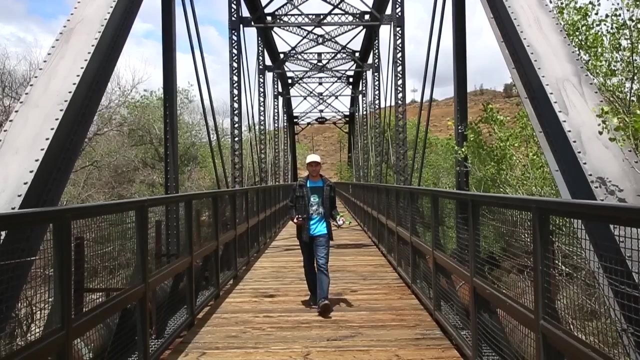 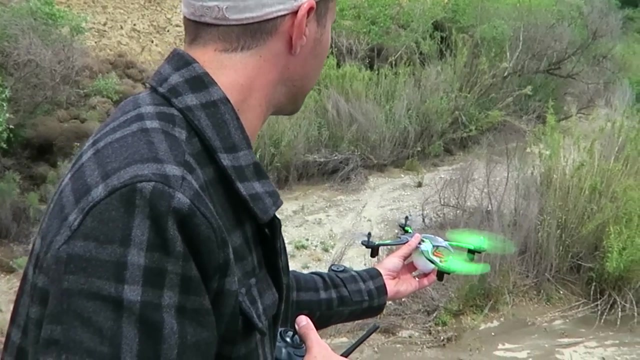 Model rocket, but without gyroscopes and control algorithms, Things can get pretty unsafe pretty quickly. So I thought of this idea where I use balloons that could deflate and then they would provide upward thrust, like before landing. but No, And As ridiculous as this might seem, it's actually not a violation for most rules, because you're not touching it once you've arrived.